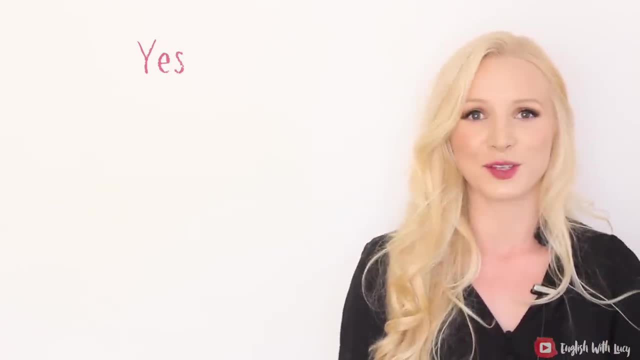 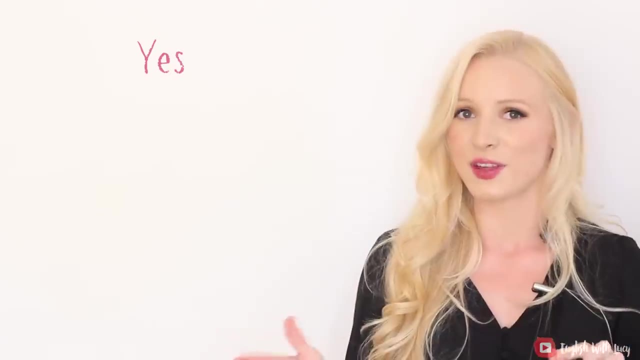 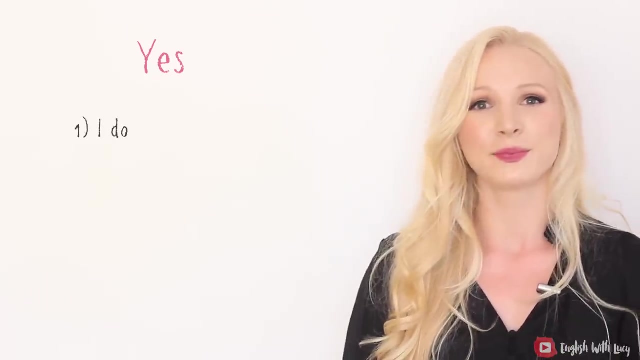 In English. we have lots of alternatives for this word, but learners of English will often find themselves just using the word yes instead of the alternatives. I have got seven for you today. The first one is this one: yep, Yep. 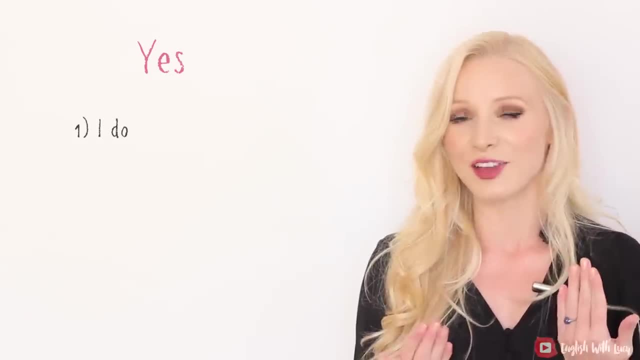 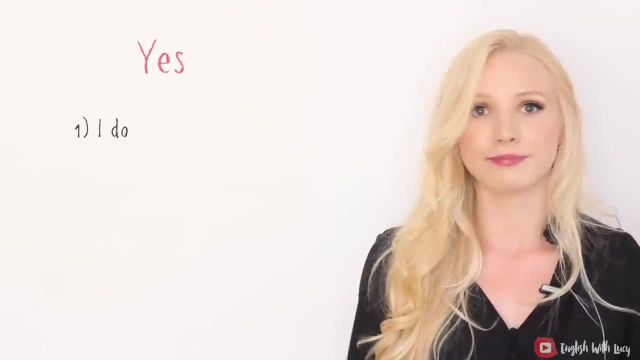 Now, this is yes. It's usually used in spoken English and it's quite informal. It's a non-standard spelling of yes and it represents the pronunciation Yep, Yep. Have you done your homework? Yep, Yep, I have. 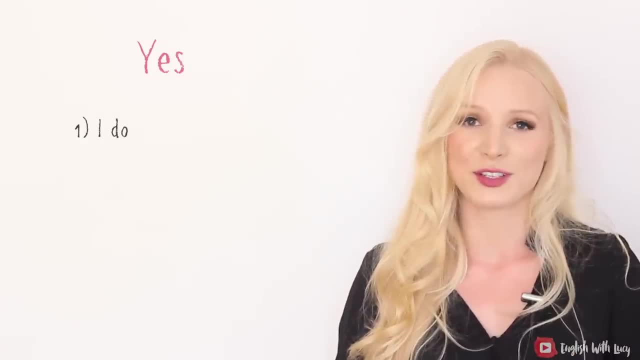 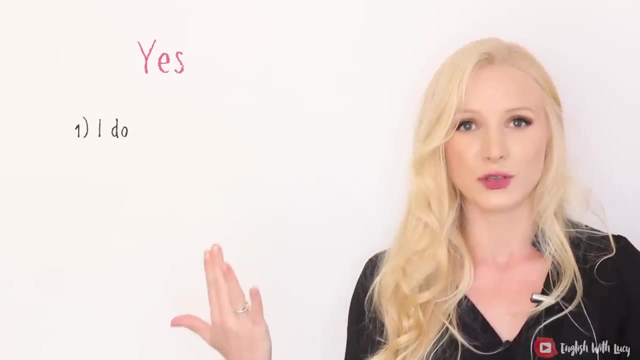 We use it all the time, especially in casual conversations, But when I was teaching students in person, I would use it and they would look at me with a face of confusion. It's not a word that you often find in textbooks. An alternative for this: yes. 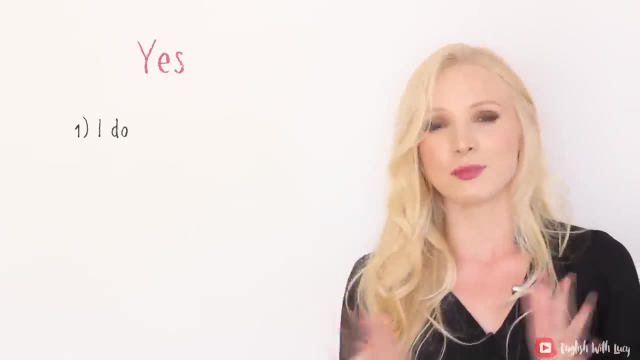 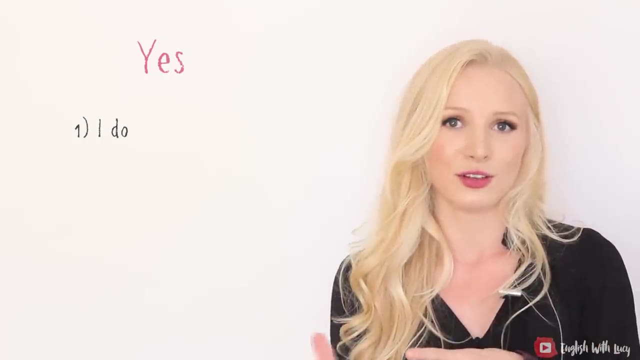 Which is used more in America. you'll still find it in Britain, but because it's a spoken word rather than a written word. this next alternative represents the American pronunciation: more It's yup, Yup. We also have number three, which is yeah. 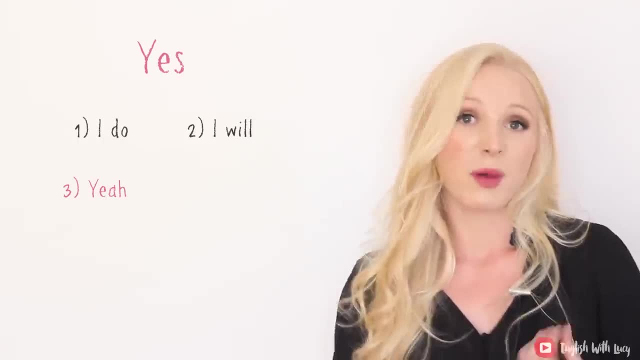 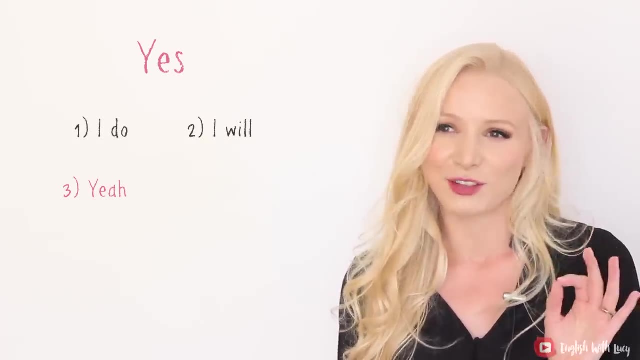 Yeah, This can be spelt in a variety of ways, but it's normally used in spoken English and it is just a casual way of saying yes. And I imagine if we did a study of any of these words, every single sentence uttered. 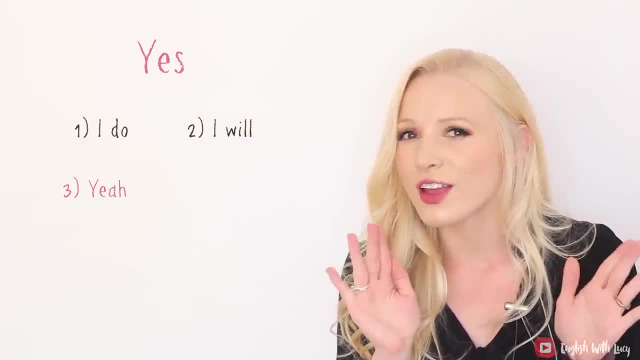 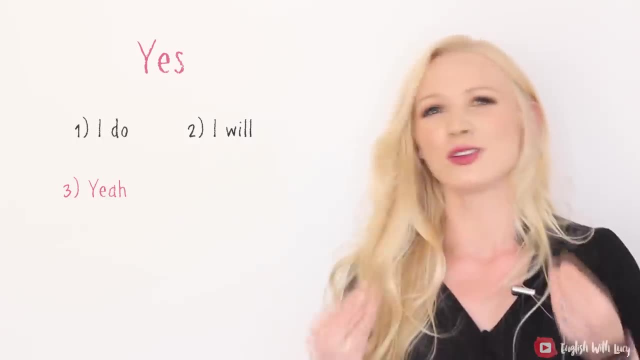 by English speakers across the world. I feel that yeah would be more common than yes. I feel that I hear it more than yes. Yes has lots of emphasis, It's more formal, Yeah is more casual and it's easier to say, in my opinion. 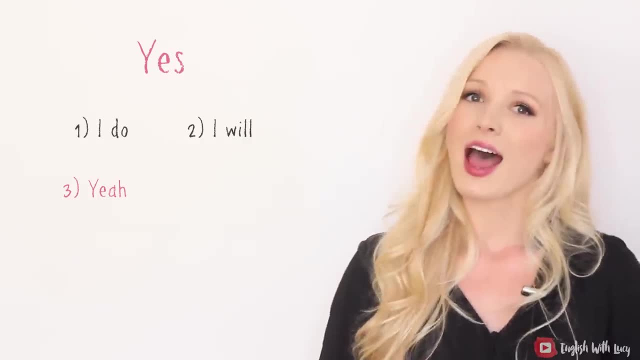 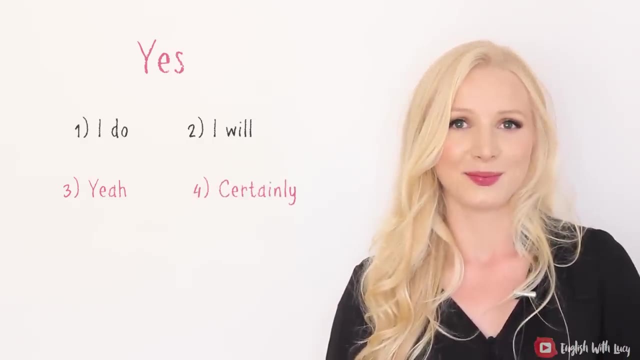 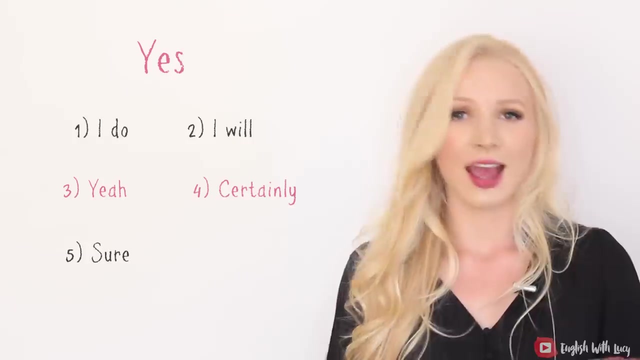 Now, number four is slightly more formal and it is used to respond usually to a request. It's certainly, Certainly, Certainly. We also have the more American version, which is sure, Sure, Can you drive me home today, Sure. 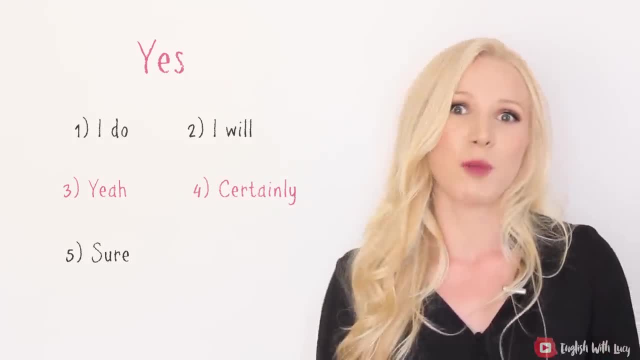 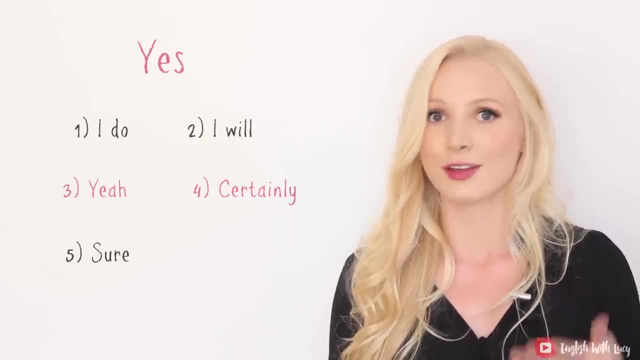 Certainly Now, because in the UK we watch a lot of American TV programmes and American films. we are becoming more used to using Americanisms like sure, so it's definitely something that we will understand and potentially use. An additional alternative, number six: 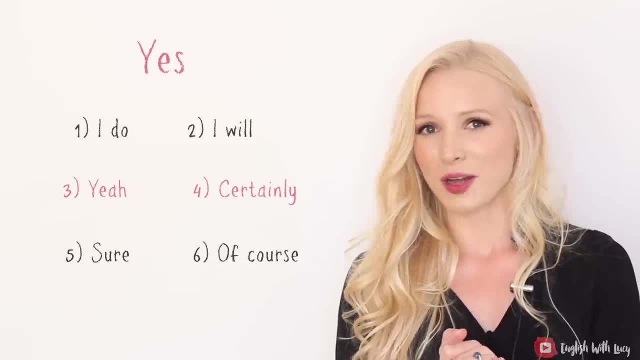 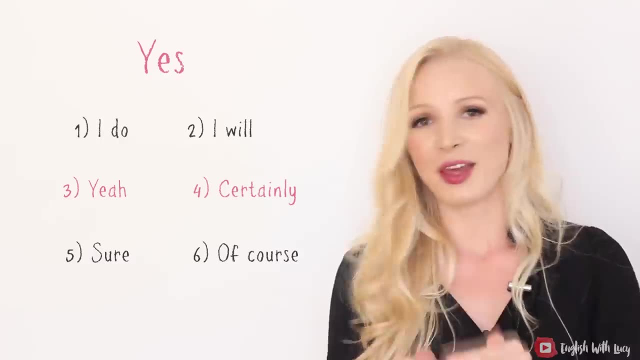 is, of course, Of course Now the last one, or should I say the last three, but I've grouped them into one. they're not necessarily a direct translation of yes, but they're used in place of yes. They are I do, I will and I have. 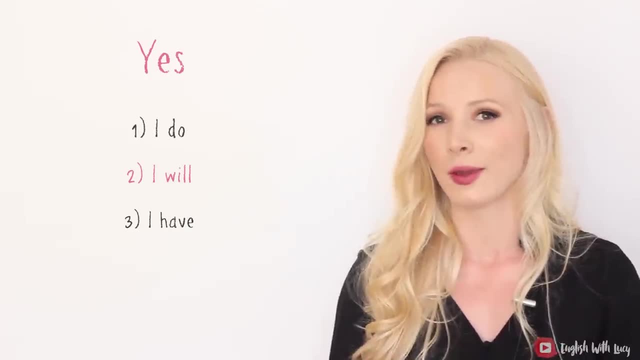 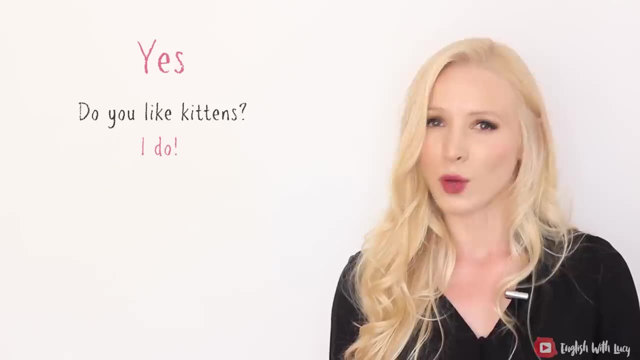 and there are many others as well. I'm talking about echoing a question, For example: do you like kittens? Instead of saying yes, you could say I do, Will you have a kitten soon? Yes, I will. Have you bought an excessive amount of cute kittens. 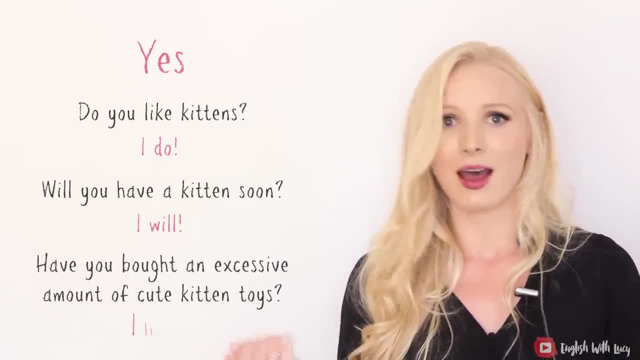 Yes or I have. I just thought I'd mention that one there. So if you find yourself saying yes a lot, you can switch it up and say something different. Now, what comes next? I'll give you a few seconds to guess. 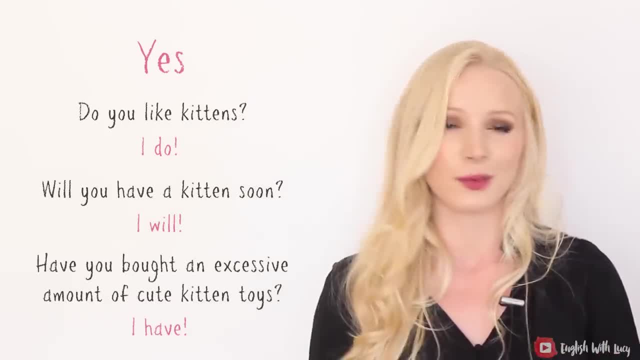 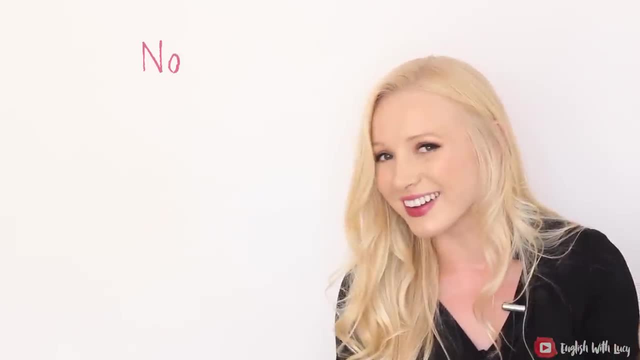 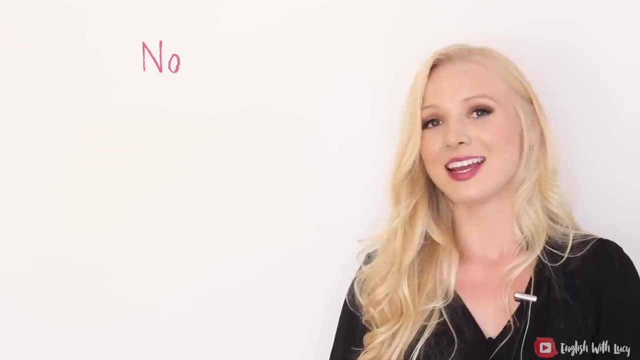 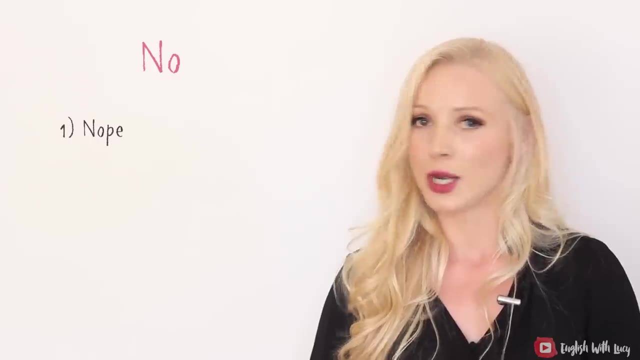 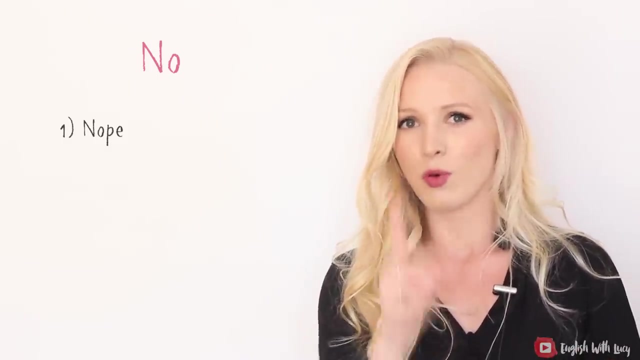 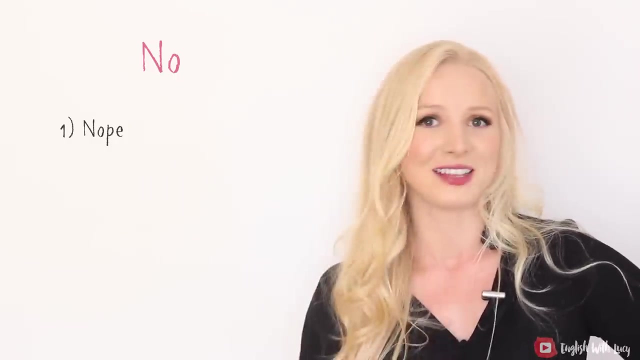 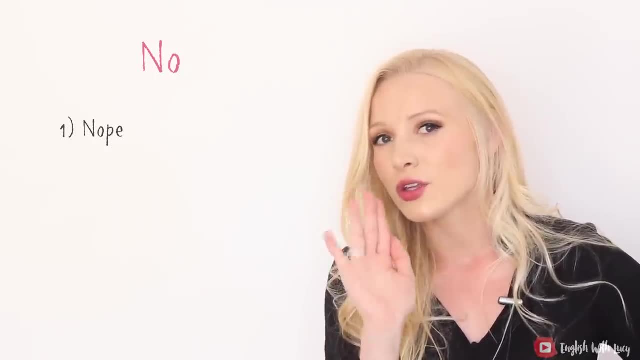 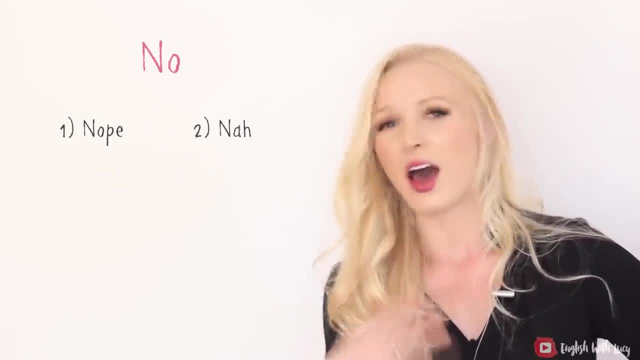 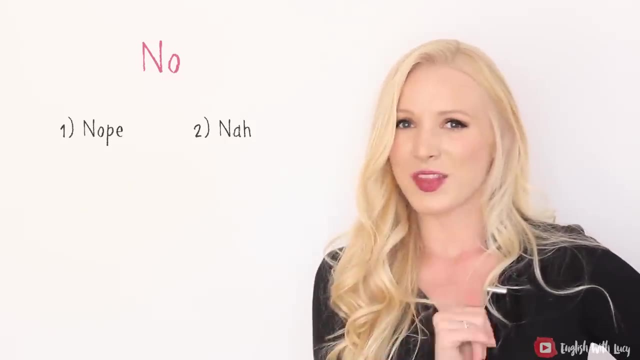 Another alternative which is potentially used more in America, and it's definitely not formal. You would not want to say this to your boss. Nah, Nah. I use this a lot. actually, i'd use it with my friends. i use it to express a bit of disgust. do you want this for dinner? oh, nah. 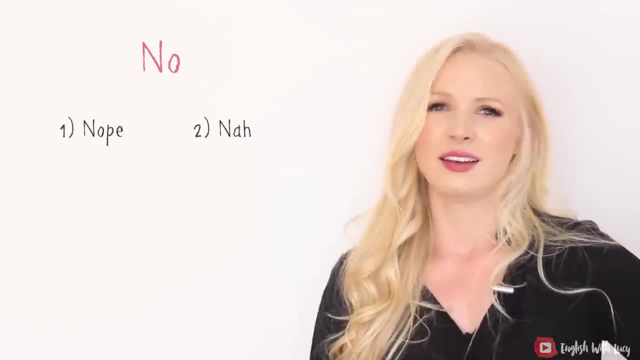 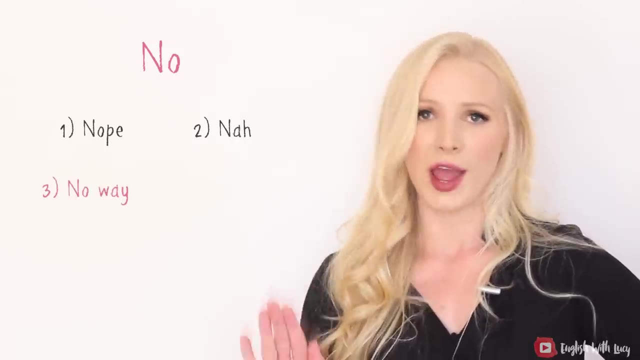 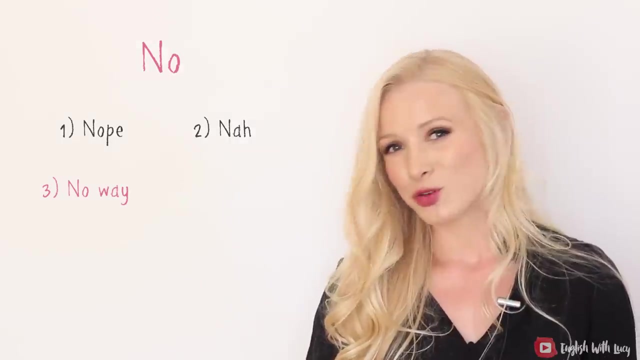 i might also use it if i'm expressing a bit of disbelief. nah, no, i don't believe that. nah, another one, which is very forceful: no way, no way, there is no way in hell that i'm going to do that. no way now. i'm not sure if you know this, but british people love to say: 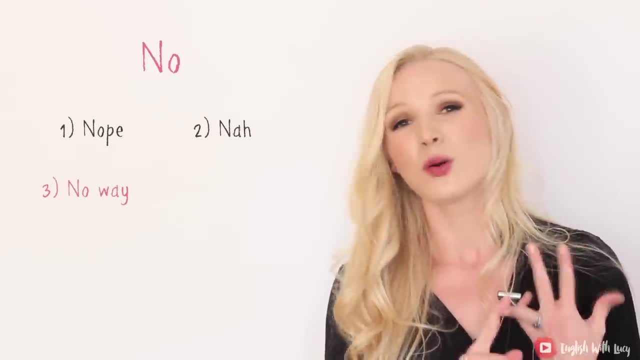 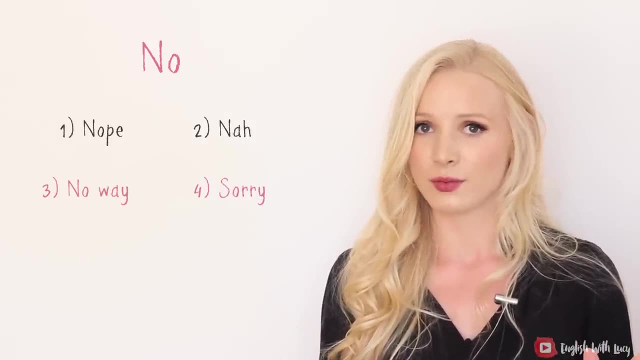 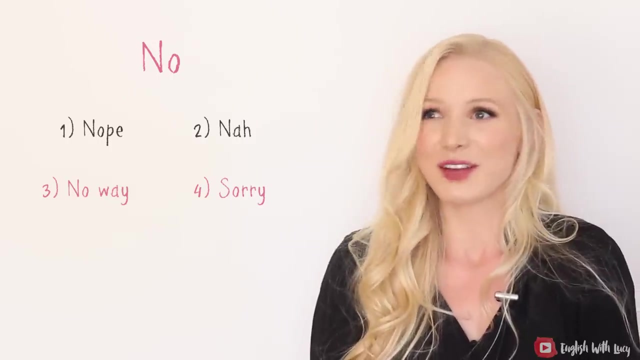 please thank you and sorry, sorry, especially all the time. so it should come as no surprise that sorry is a perfectly fine alternative for no. this is global, but especially in britain. are you coming tonight? sorry, don't even have to say no, just a sorry will do something that's slightly less. 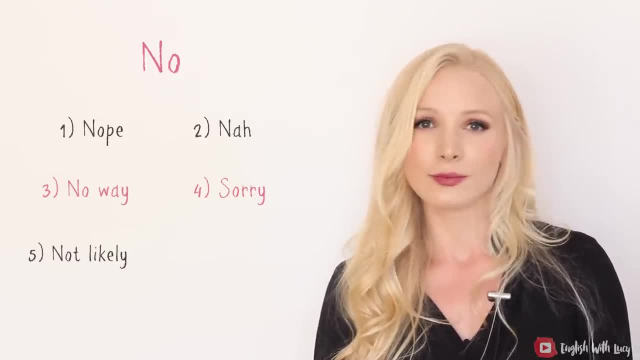 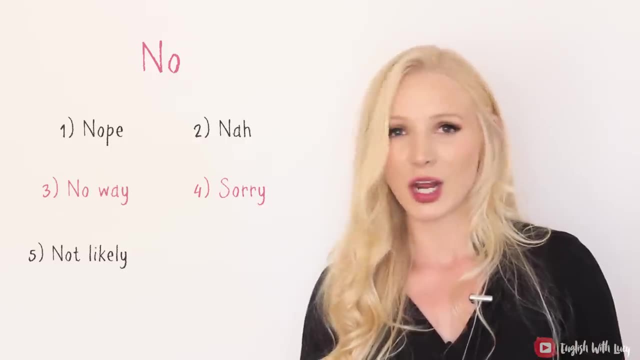 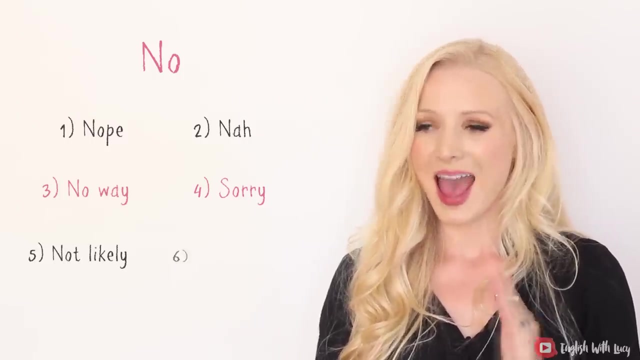 strong, is not likely, not likely, rather than saying it's not likely, just not likely will do. do you think you'll get a promotion this year? not likely, no, i don't think that i will get a promotion this year. now another really forceful one. we can say absolutely not or certainly not. i love that word and i'm noticing. 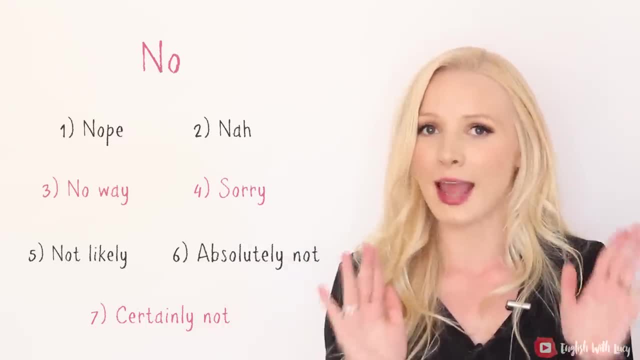 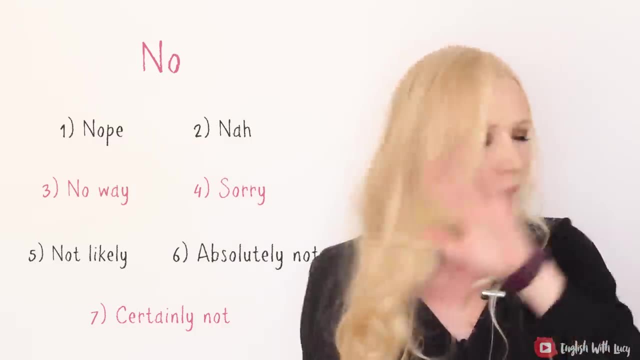 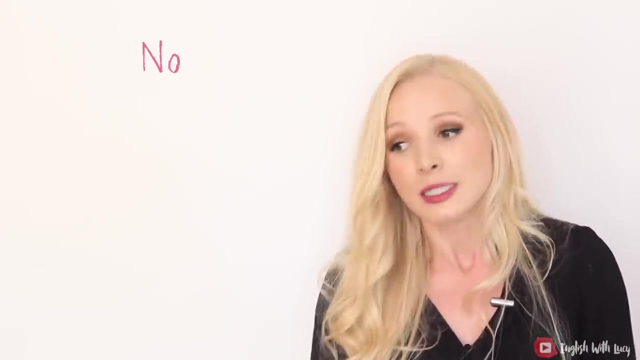 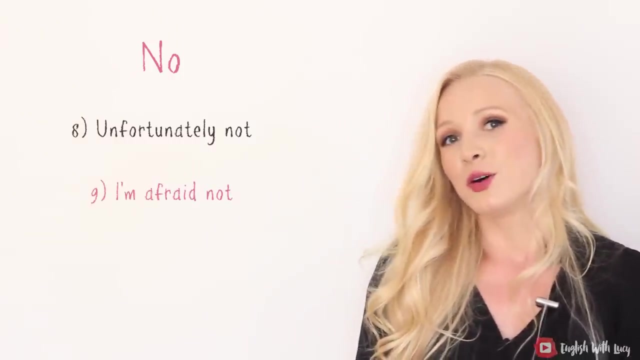 it growing in popularity. at the moment, everyone seems to be saying absolutely. so get on board the absolutely train. absolutely not. will you go out with him again? absolutely not, certainly not. if you want to express no in another apologetic way, we have, unfortunately not, unfortunately not, or we also have, i'm afraid not, i'm afraid not. 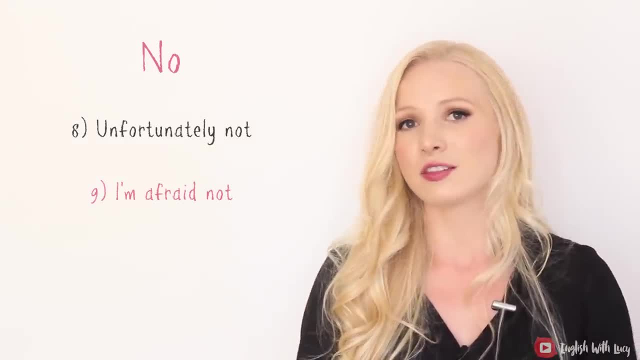 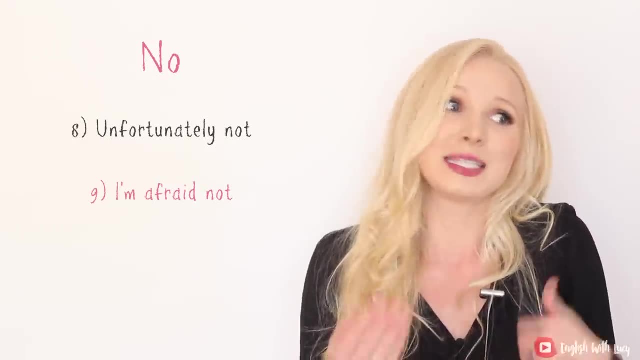 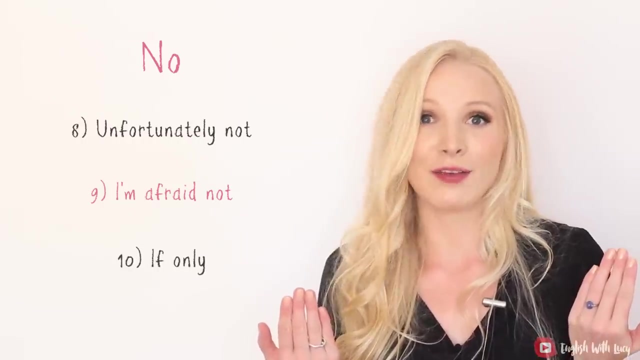 and don't get this confused, because to be afraid of something is to be scared of something. but if i say i'm afraid not, it means i'm sorry. you know, i'm scared to tell you this because i'm so sorry about it. but no, we also have, if only, if only short, for if only i could. 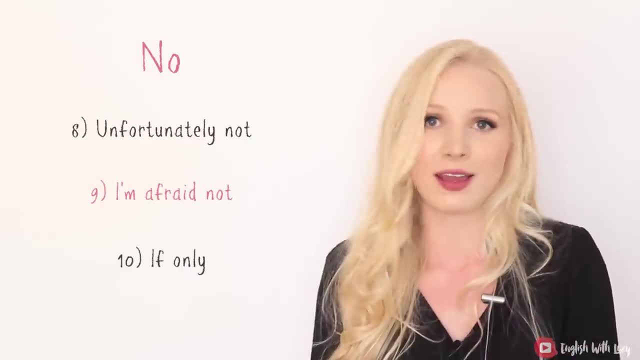 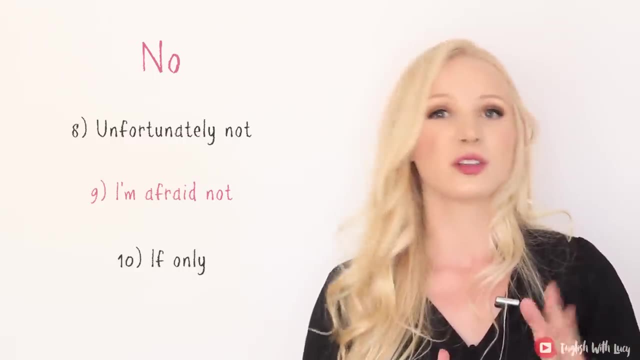 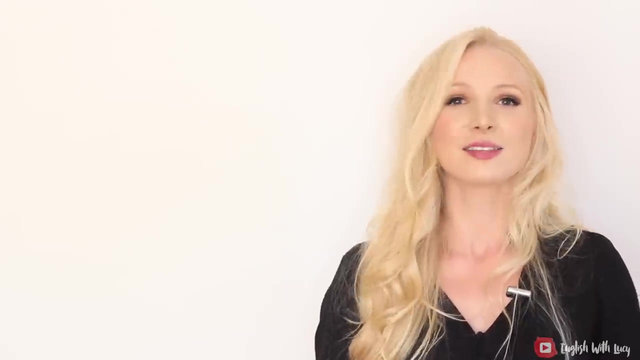 if only, if only i could, but i can't. it's implying that you can't. and finally, one to use if you're offered something or you're offered an experience and you want to decline it. i'll pass short, for i'll pass on that. no, thank you. right, let's move on to britain's favorite word: sorry, i've got. 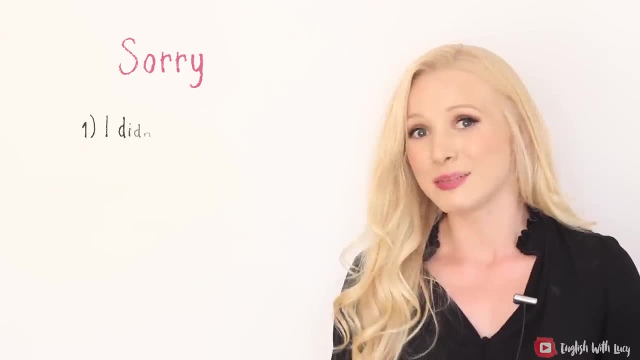 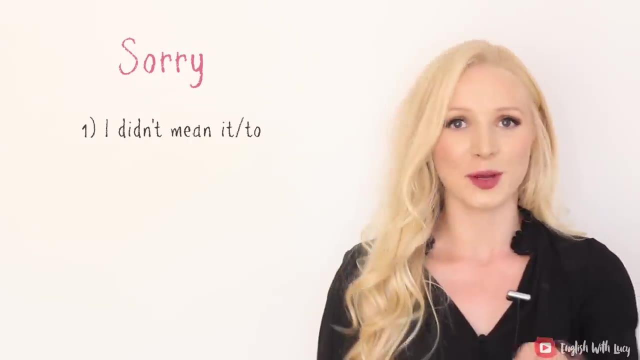 five alternatives for you. the first one is: i didn't mean it or i didn't mean to most of these. These can be used in conjunction with sorry, So don't worry, Brits watching you can still use your favourite word: I didn't mean to run over your toe. 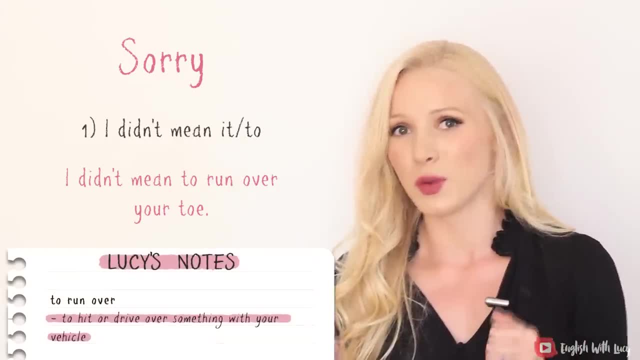 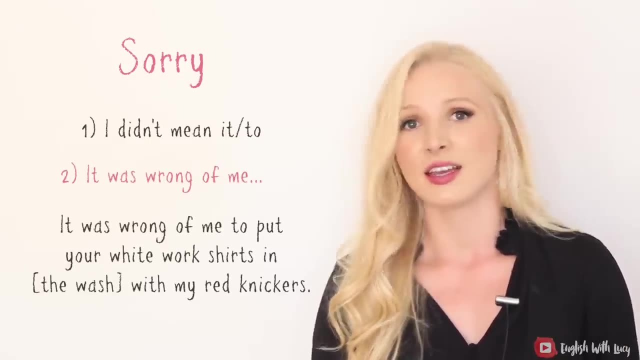 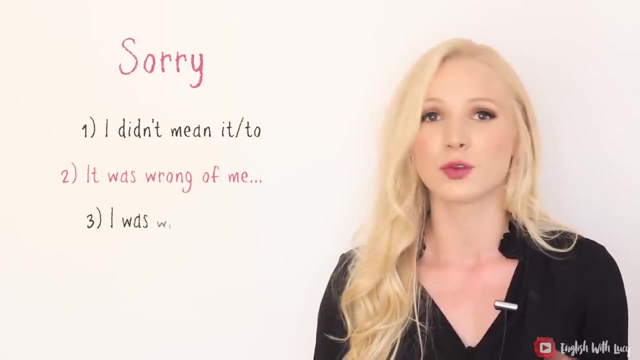 To run over something implies that you have gone over it with your car wheel. Another one: it was wrong of me. It was wrong of me to put your white work shirts in with my red knickers. Got pink work shirts now. Alternatively, you could say I was wrong too. 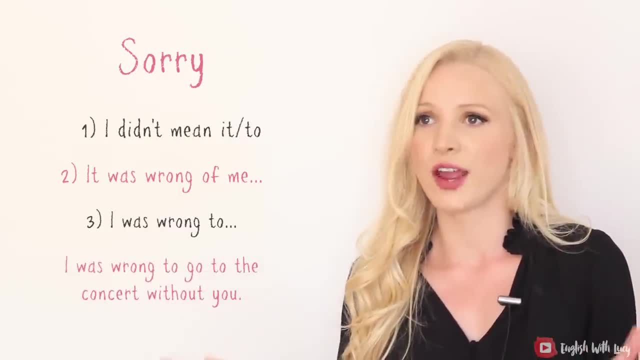 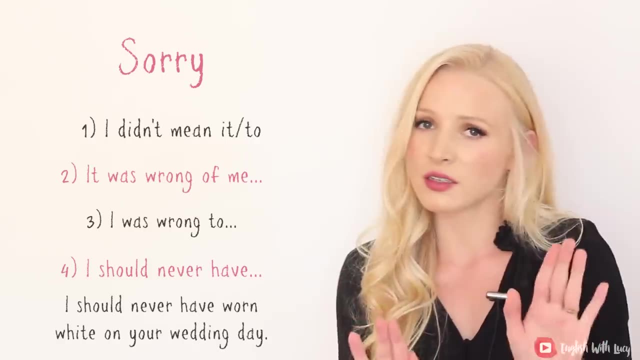 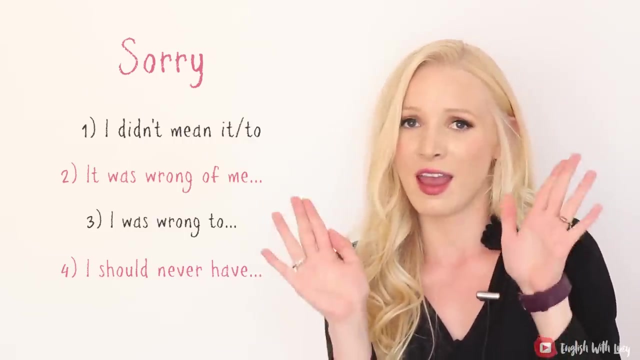 I was wrong to go to the concert without you, to go and see your favourite band without you Also, we have. I should never have. I should never have worn white on your wedding day. True story: I didn't wear white, but I went to a wedding and a girl was wearing. 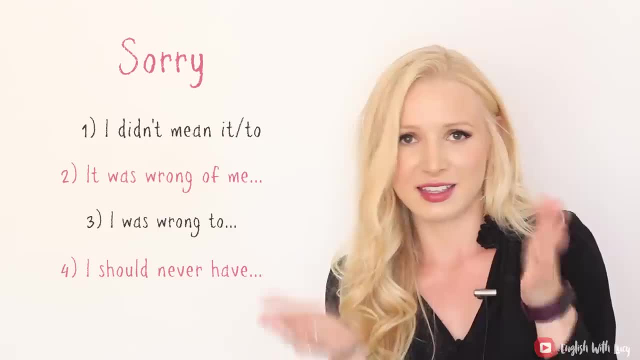 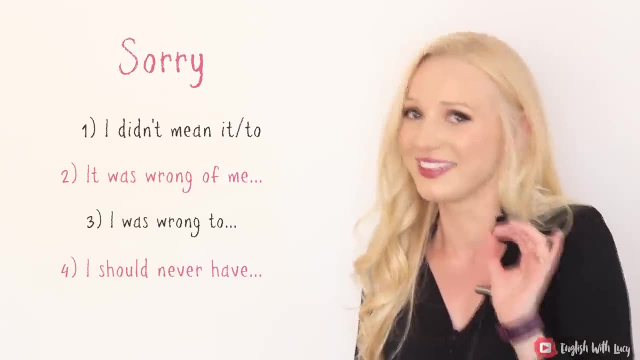 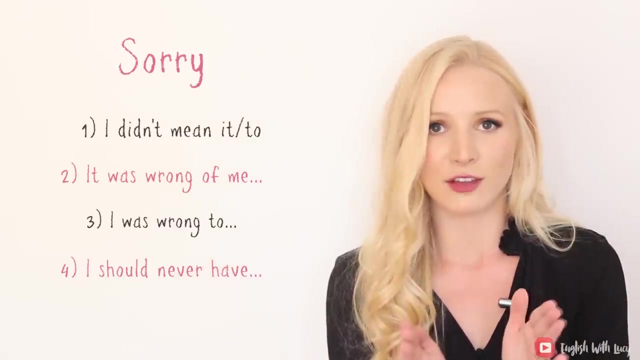 a white bridal style dress. Is this okay in your culture? Let me know, because it's not okay in ours. Didn't say anything, just judged silently. Now the last one. this is definitely an Americanism. It's come over to the UK and it's very, very casual. 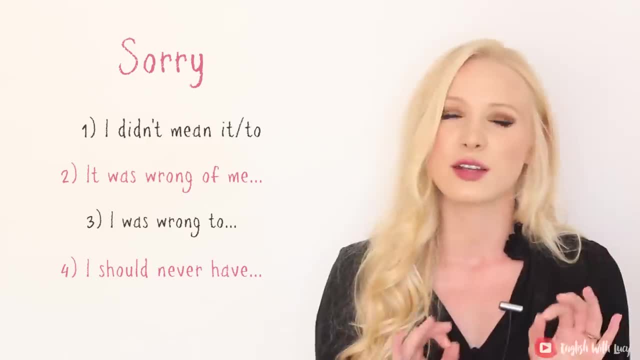 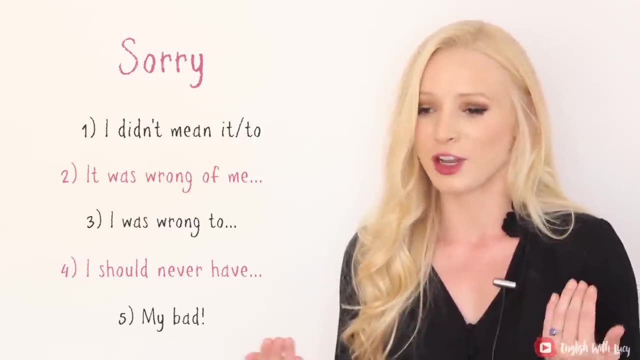 and can sometimes be considered obnoxious if used in an incorrect situation. so be careful with it. But it is my bad, my bad Now. I remember being a young child and hearing this on programmes like Friends and I didn't really understand what it meant. 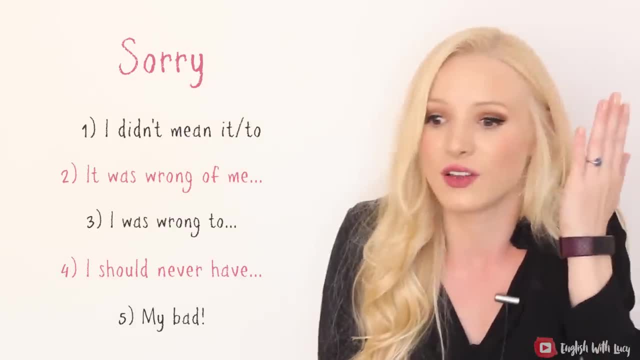 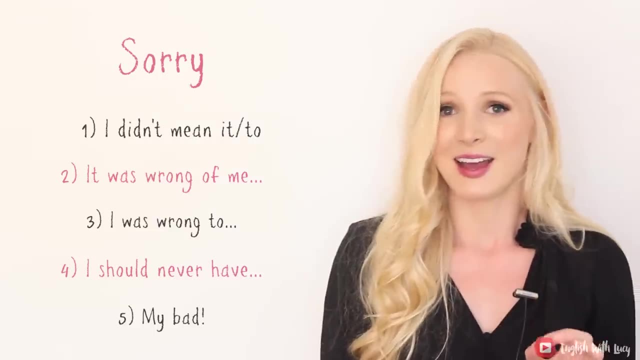 I was always taught to say sorry, of course because I grew up in Britain and it's our favourite word, But I remember hearing my bad and thinking you're bad like you are bad. No, my bad. It's a very casual, fairly impolite way of saying sorry. 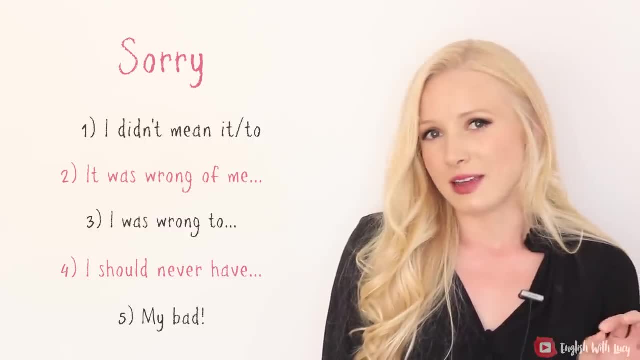 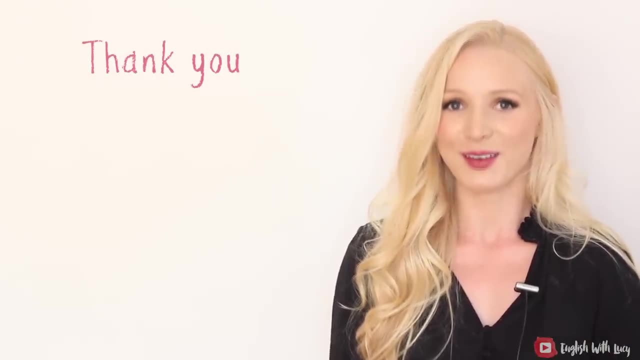 It's okay to use it with your friends and if it's not a serious mistake, Okay, let's move on to thank you. thank you. I have got eight alternatives for thank you. Lots to do here. The first one is: you're a star, you're a star. 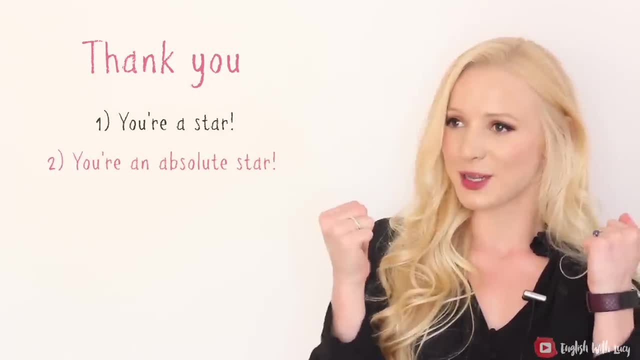 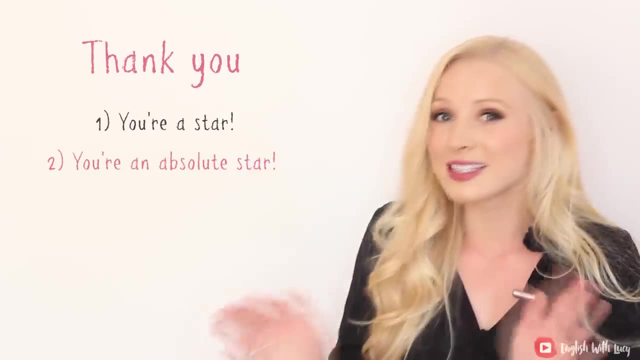 Or you're an absolute star. we're using the absolute word instead of saying thank you, thank you, we're just telling someone that they're so wonderful and we appreciate them so much. Very similar is: you're a lifesaver, You're a lifesaver, So that means that somebody has 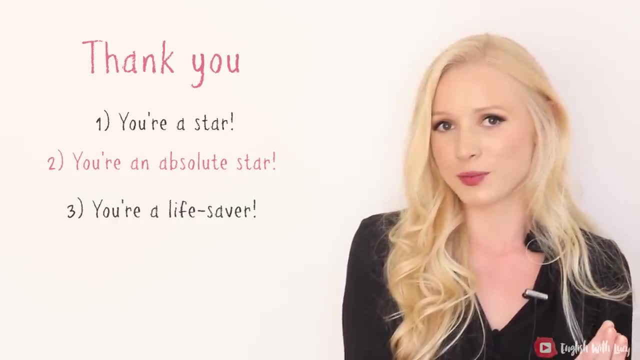 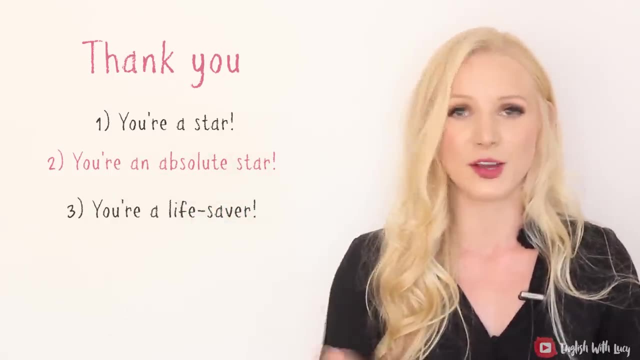 done something that has saved you a lot of trouble. Maybe you left your phone on a train and somebody managed to get in contact with you and give it back to you. You're a lifesaver. You've saved my life, You've brought me my smartphone back, and that is my life. 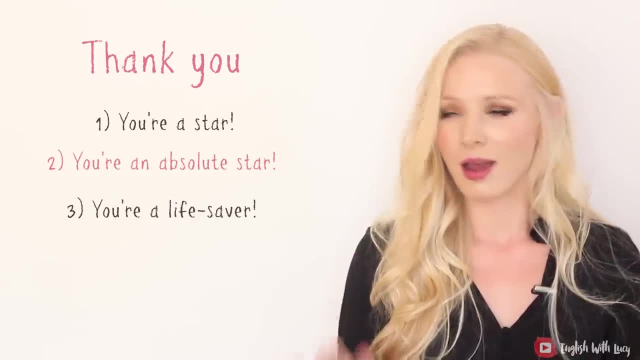 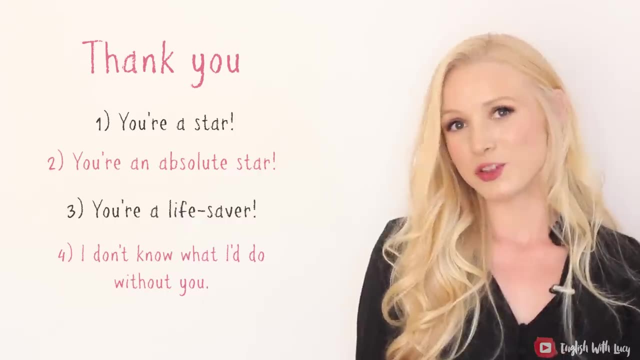 That's another way of showing that you really appreciate someone. I don't know what I'd do without you. I don't know what I'd do without you. Very similar to lifesaver, Another one which is a good way to respond to a compliment, because 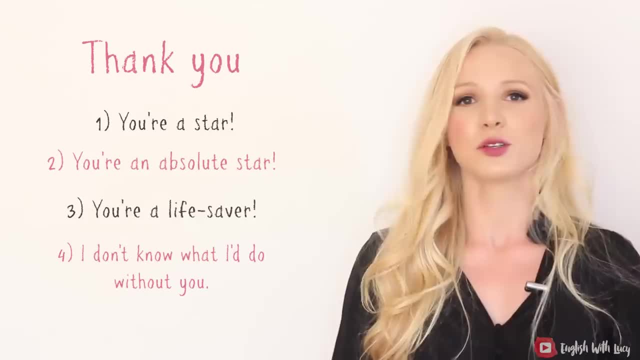 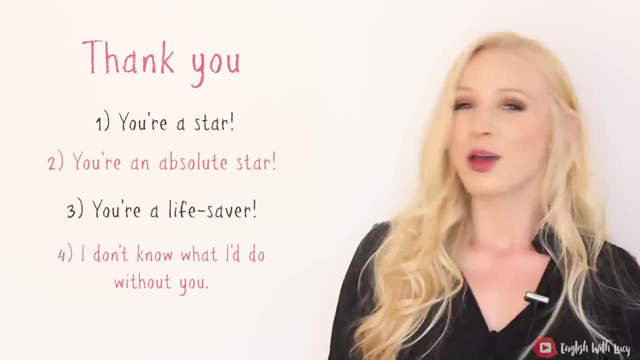 if you're lucky enough to receive lots of compliments, you might find yourself saying thank you, Thanks, Thank you, Thanks all the time, And that's a wonderful problem to have. but another phrase that we can use is: I appreciate that. I appreciate it. 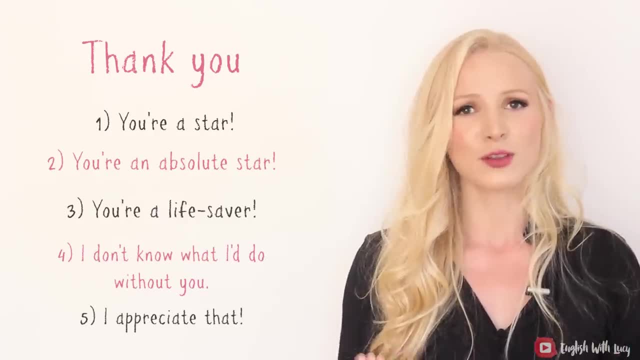 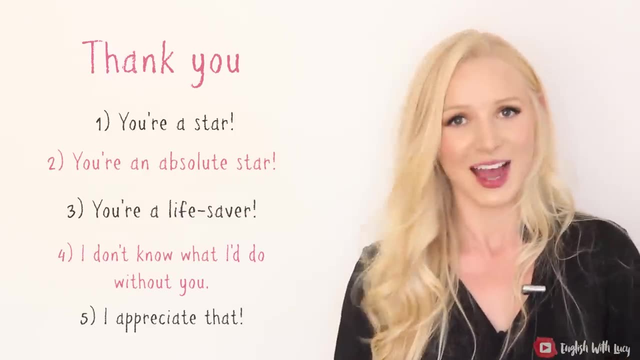 I appreciate that. Yeah, it's a nice one. So next time you receive lots and lots of compliments, you can switch between thank you, I appreciate that. Thanks, I appreciate it. You're just so lucky to have me, aren't you? 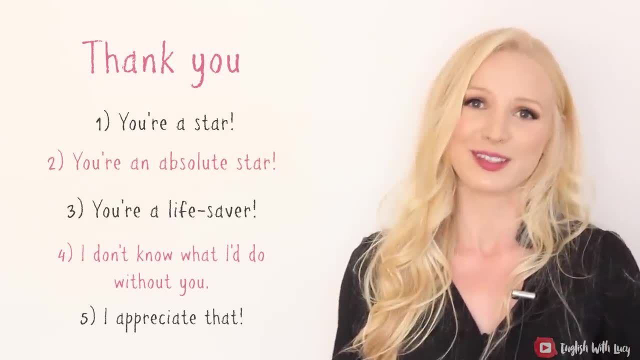 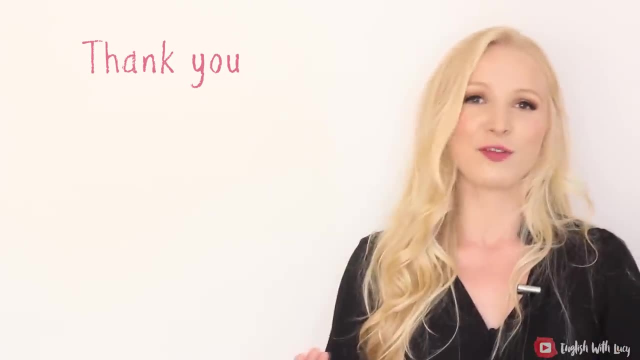 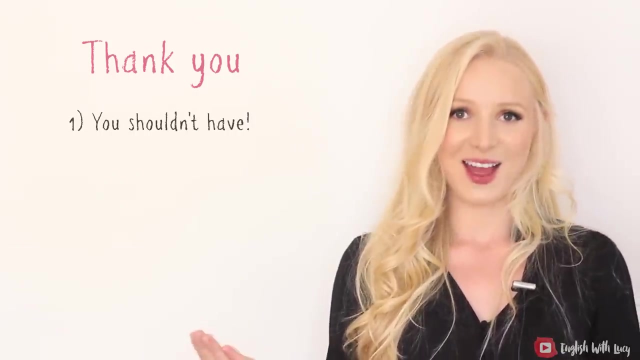 I have equipped you for your next influx of compliments. You're welcome. Now, something you can say: if someone has made an extra effort for you, if they've gone above and beyond, that means to make an extra effort. you can say you shouldn't have, you shouldn't have. 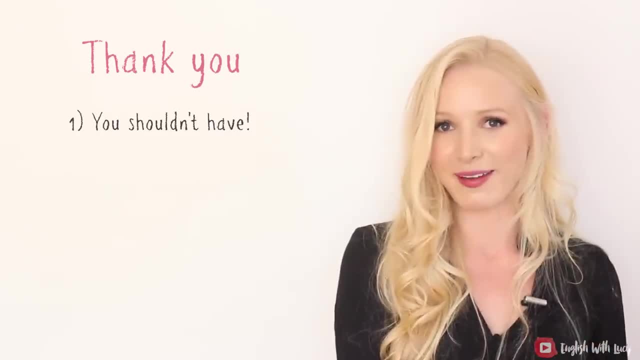 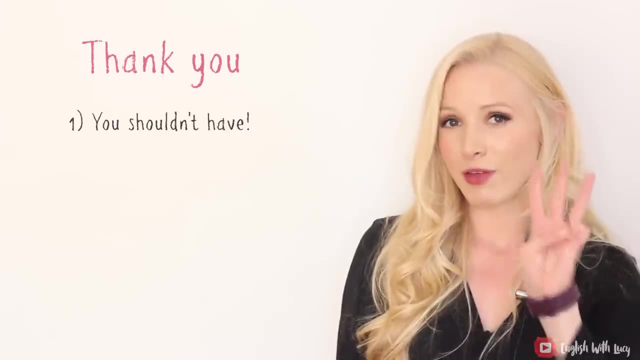 And this doesn't literally mean you shouldn't have done something. It's obviously done with a smile. It means you shouldn't have gone to so much effort. Thank you so much. Finally, we have three informal ones. One is extremely British. 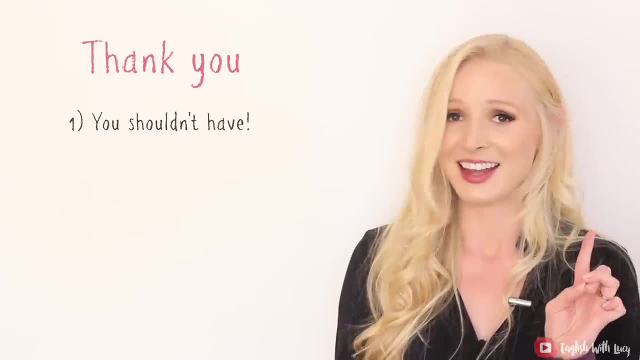 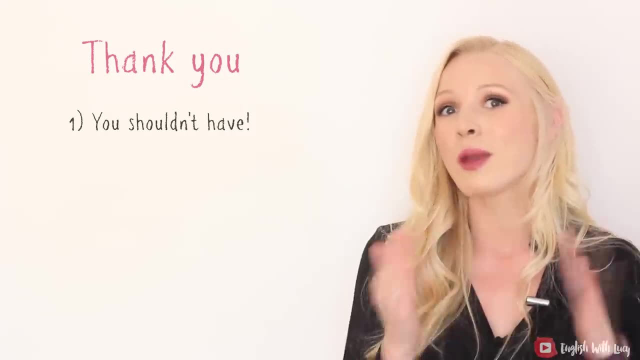 And there was actually a study the other day- the other day I mean a couple of years ago- in a very unreliable newspaper, but I enjoyed reading it saying that this word has now replaced thank you. It is cheers, Cheers, And this is typically something we say. 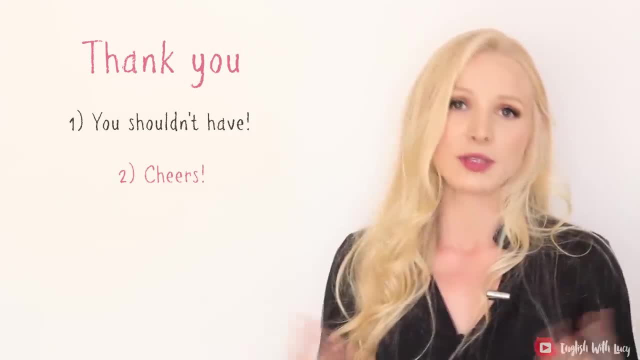 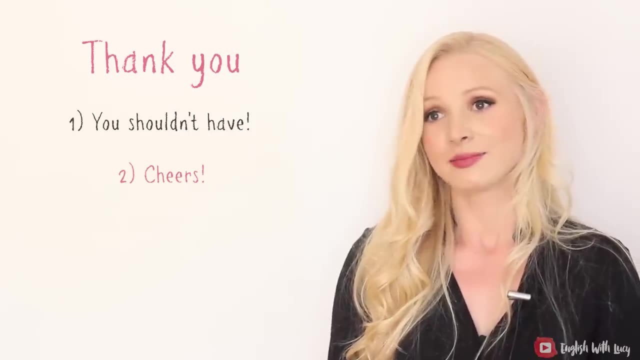 when we bash our drinks together before drinking them, but now it's something we use instead of thank you, Cheers, Cheers, mate. Thank you for that. Another one which I don't like, and I've said this before in a video. I don't like it. 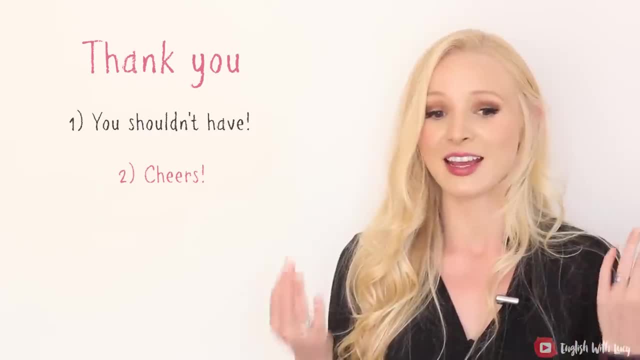 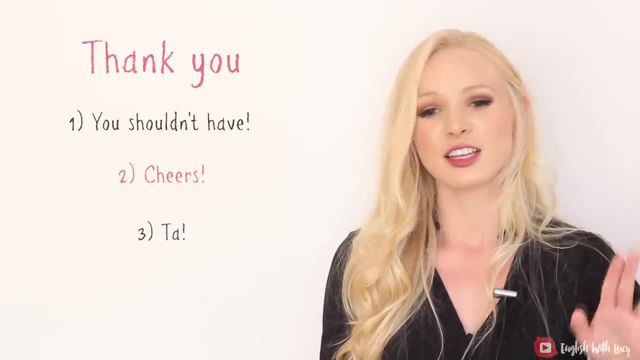 At nurseries and at schools they encourage the children to say ta instead of thank you, because it's easier to say. But when someone says ah, ta, ta very much, I just think it sounds like they're not putting in enough effort. 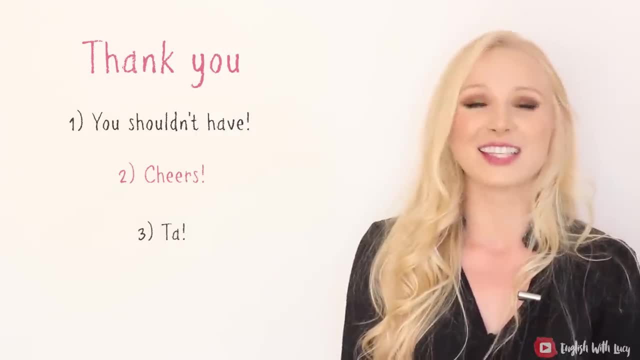 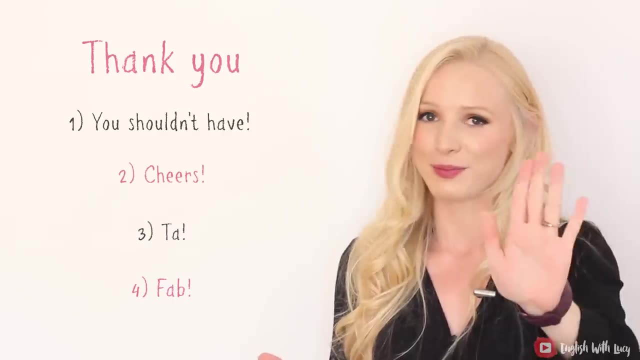 but maybe I just need to get over myself. And then the last one is fab, short for fabulous. It's just a way of saying great, thank you so much, Fab. that's fab, Okay. lastly, onto overused word number five. 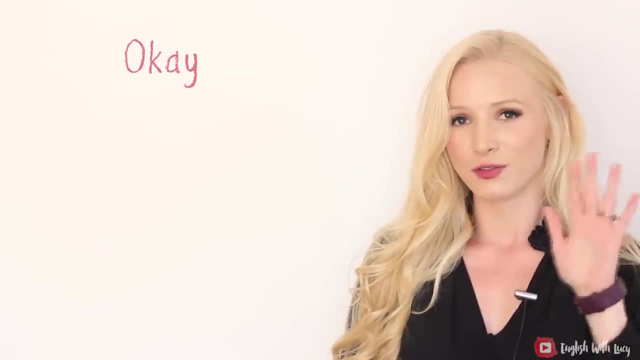 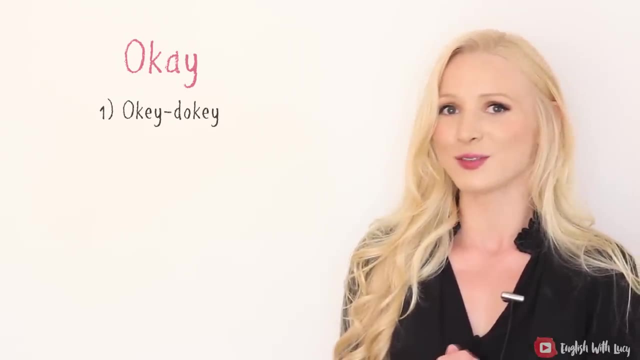 It's okay. Okay, I have got five here for you. The first one is okie dokie, Okie dokie. or is it Ned Flanders from The Simpsons that says okie dokie? Maybe don't say that. Well, you can. 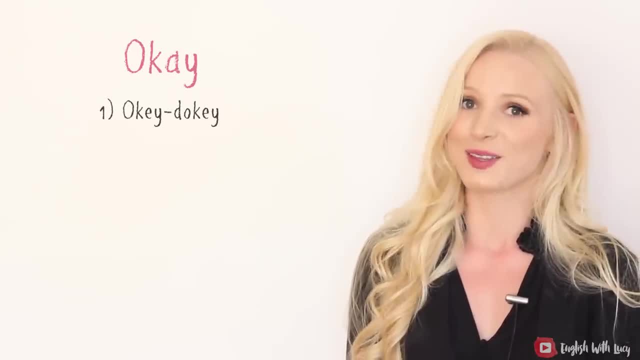 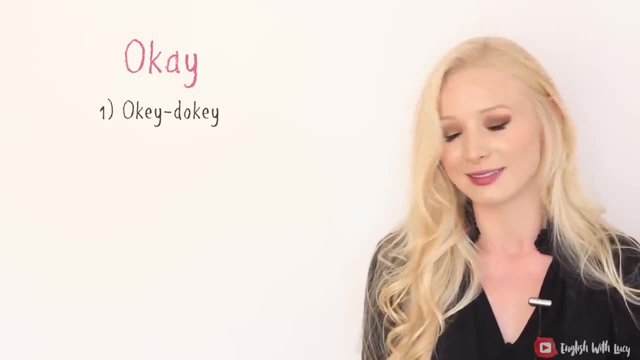 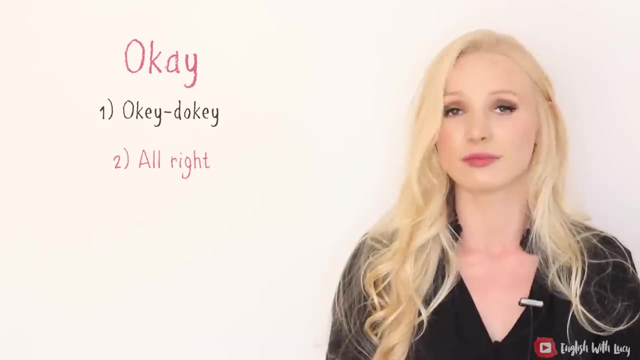 Okie dokie is very common. It's definitely something that's informal. Use it amongst friends, Potentially. don't write it in formal academic writing. Definitely don't use it in formal academic writing. Another very plain and simple alternative is: all right. 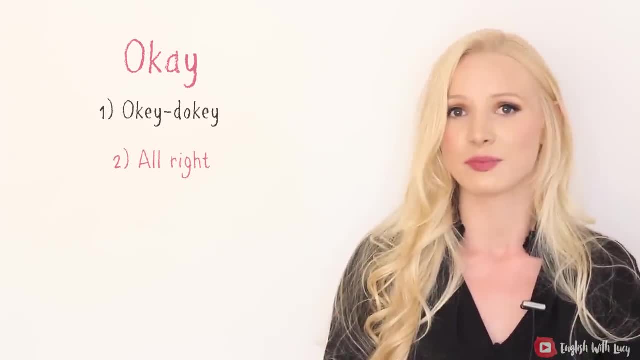 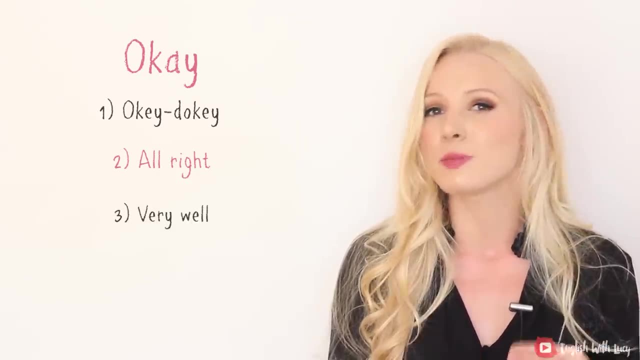 Right, okay, all right, They are almost exactly the same. We also have very well, very well, which almost implies a little bit of displeasure. Very well, if that's what you want. Next we have righto righto. 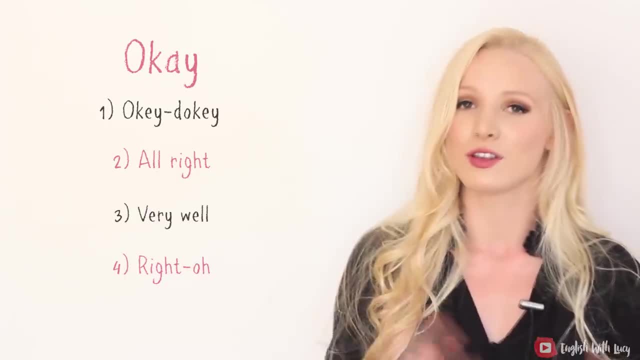 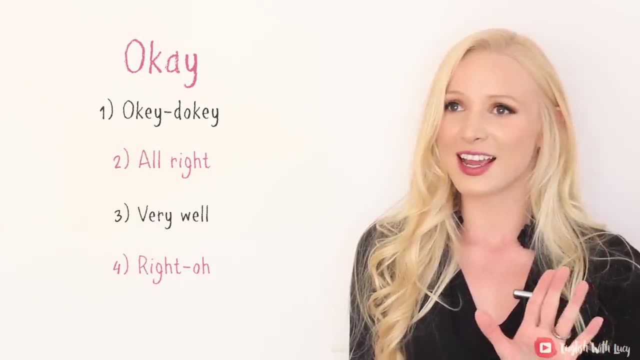 And this is one that has come from my fiance. I asked him just before writing this script if he can think of any other alternatives for okay, And he said: righto, And this is definitely one that is used by the older generation, I think. 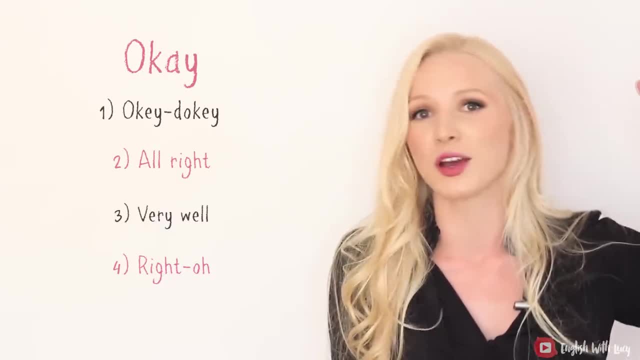 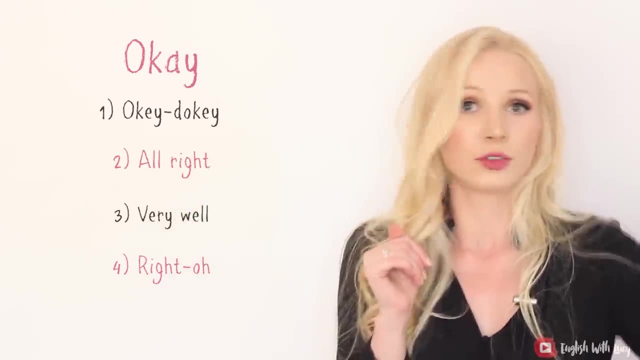 But I think it's a lovely one, And these older, kind of more old fashioned words do come back in fashion. If I were to say to him: oh, by the way, my mum's coming over for lunch, righto Good, okay. 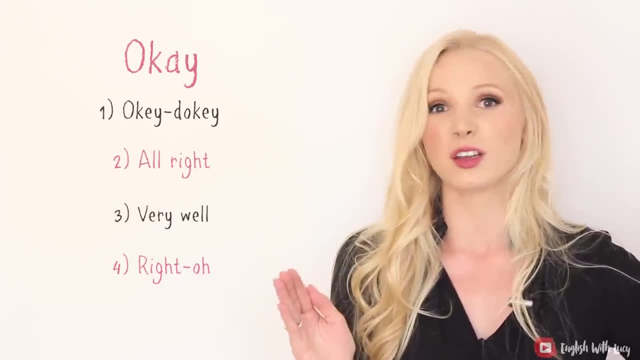 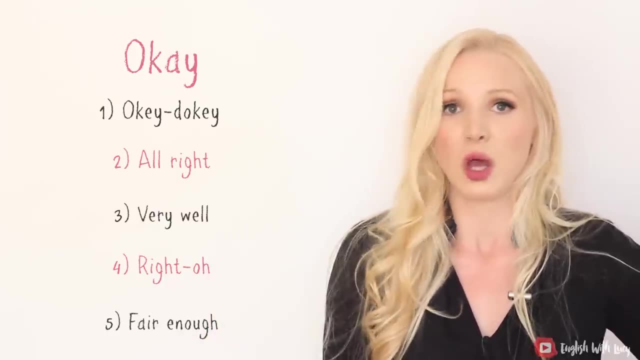 And the last one, one that is very commonly used in Britain, when we don't want to express, you know, positive or negative emotions about something. Fair enough, fair enough, Okay, I have no feelings about this, Right? that was it for today's lesson. 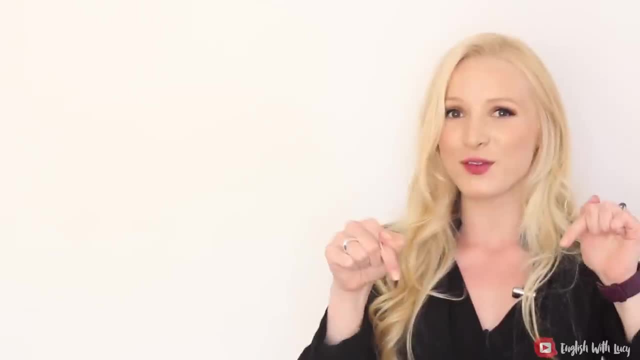 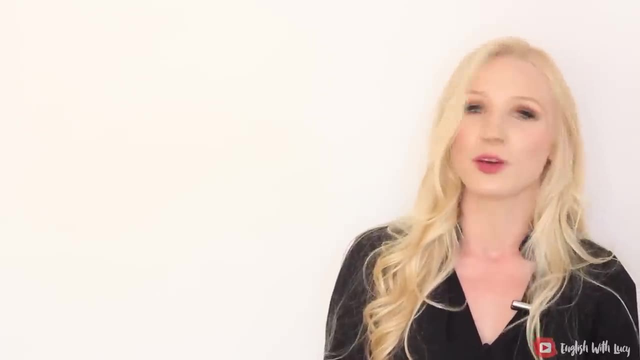 I hope you enjoyed it and I hope you learnt something. Please feel free to share any other alternatives that you can think of or any alternatives that you use in your own language that might not necessarily translate into English, but might be interesting. I'm always interested in where you're from. 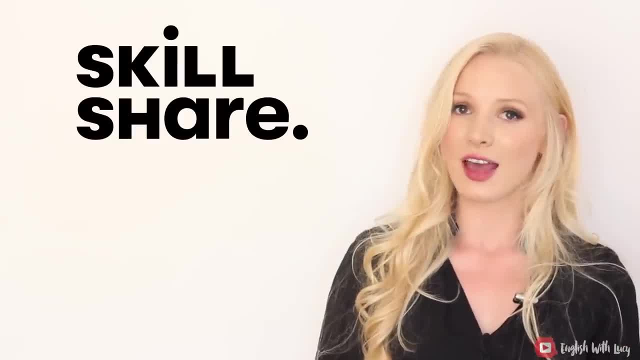 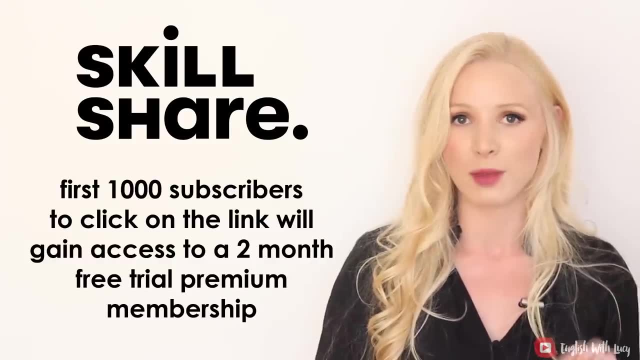 and what kind of words you use. Don't forget to check out Skillshare. The first 1000 of my students to click on the link in the description box will get a two month free trial of premium membership. And don't forget to connect with me.